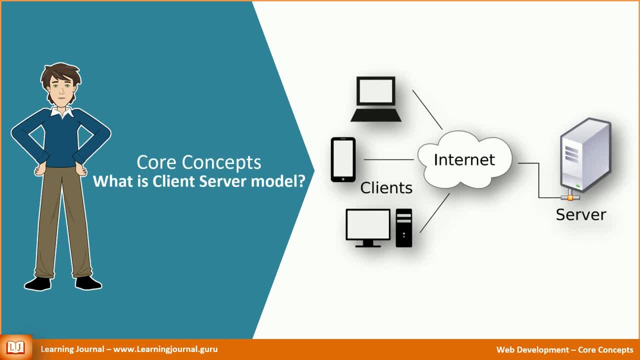 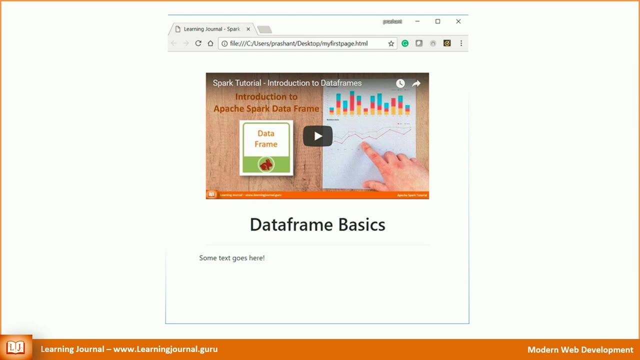 machine. However, no one else on the planet will be able to access your website until you take it to the internet, right? So let us talk about taking a website to the internet. I have this simple web page. This page is my website. It is not that great, but this is what I have. How can 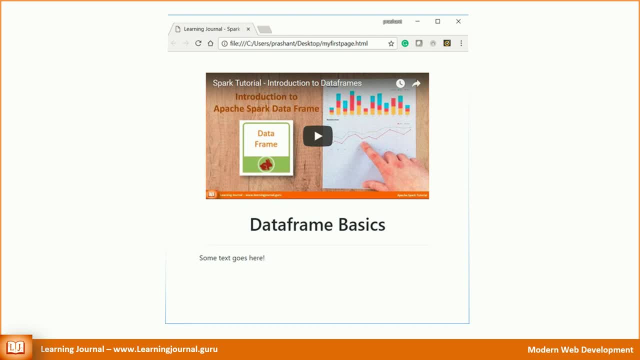 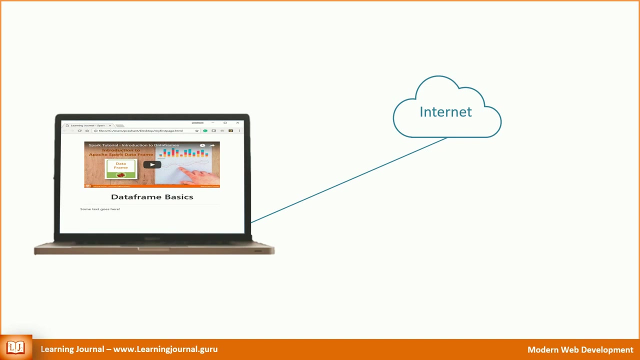 I take this website to the internet. What do I need? Just think about it. Tell me at least one logical thing. Yes, you are right. The first thing that I need is a computer with an internet connection. We all have such computers, but unfortunately that is not enough to make my 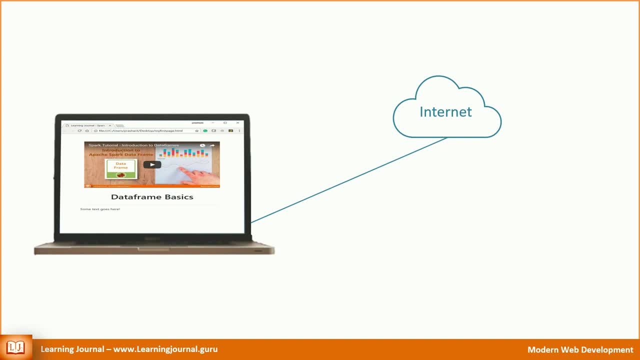 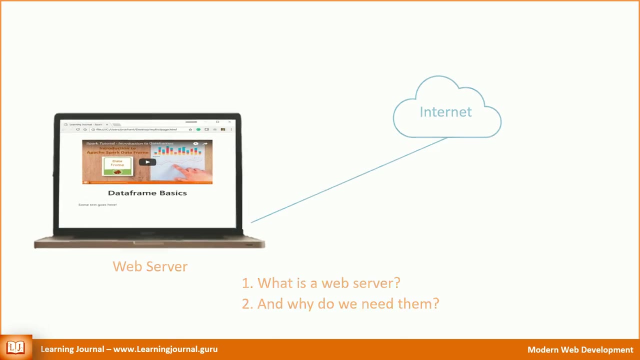 website available over the internet. I need at least one more thing, that is, a web server. I am sure you are wondering with some questions: What is a web server and why do we need them? Let us try to understand the need for a web server and then we will try to define a web server. Suppose. 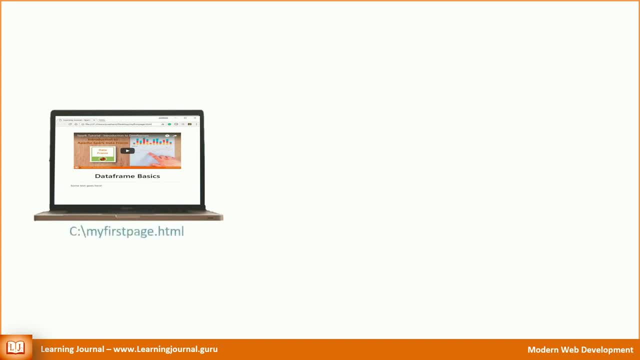 I have a single page on my laptop. I saved it at the following location. Now I want to make it available to the internet, So I connected my laptop to the internet. As soon as I connected my laptop to the internet, I estaban roads in my system and the internet connected my laptop to. 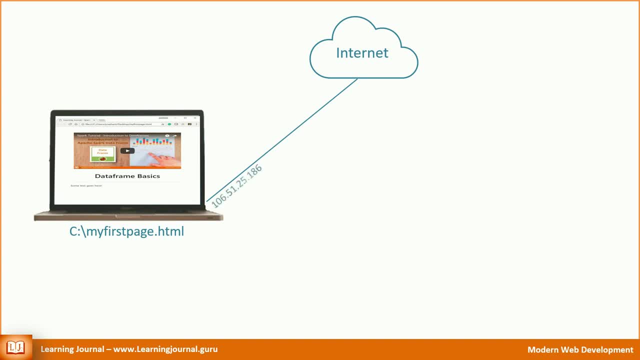 internet. my internet service provider will assign a unique IP address to my computer. On the other side. you are sitting somewhere on this planet with another computer. You also connected your machine to the internet. Technically, there is a connection between our computers. 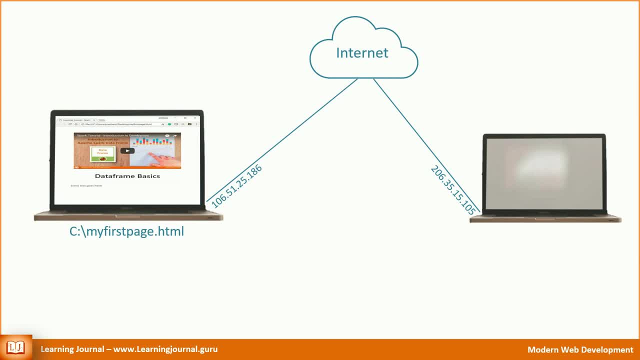 And both of them have two different, unique IP addresses. right, You should be able to start a browser on your laptop and type my website's address, And there comes a series of problems. The first problem is this: What is the address of my website? 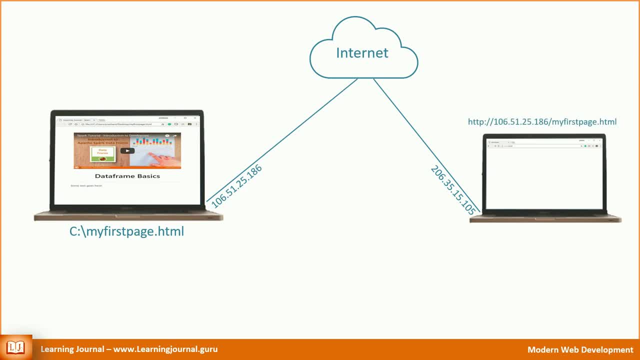 Well, it could be the IP address of my laptop and the file name. Let us assume that the first problem is solved. Now you can type this address into web browser. The browser will look at the IP address. The IP address is like a telephone number. 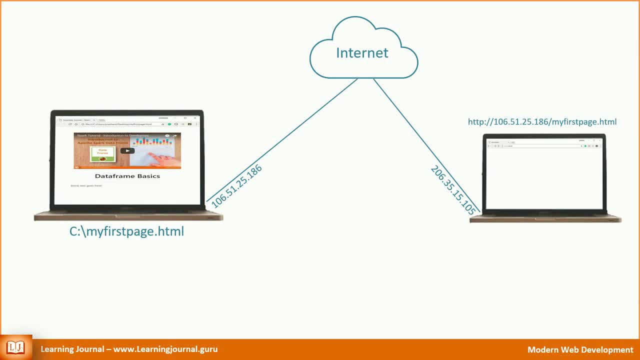 If the browser knows the IP address it can send some data to the computer with that address right. So the browser sends a request to my computer asking for the myfirstpagehtml file. That request reaches my computer And there comes the next problem.